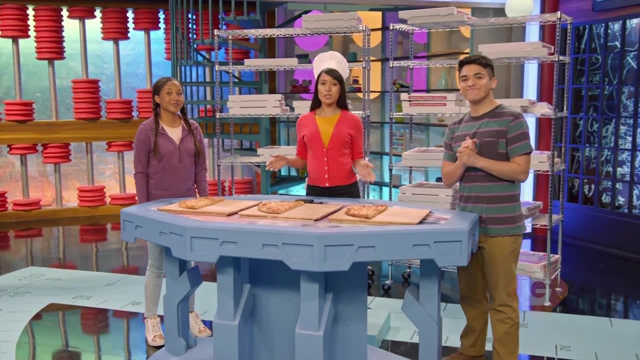 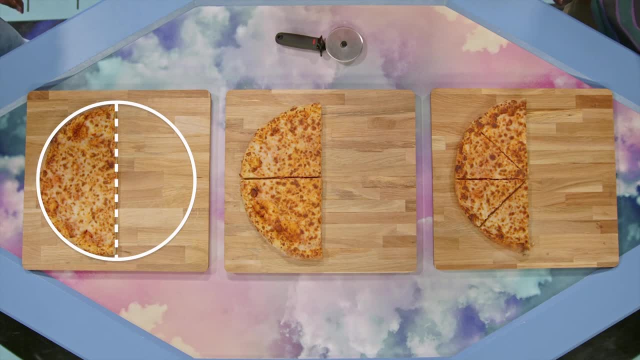 Earlier today, each of us ate some pizza. Let's see how much pizza we have left. My pizza was cut into two equal pieces and I have one left, So we can represent this as the fraction 1: 1⁄2.. 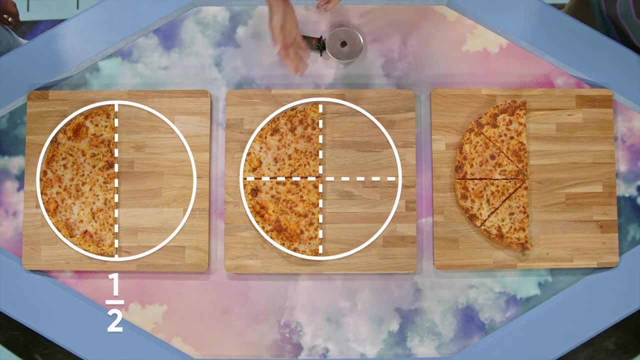 My pizza was cut into four equal pieces and I have two pieces left. We can represent this as the fraction 2⁴. My pizza was cut into eight equal pieces and I have four pieces left. We can represent this as the fraction 4⁸. 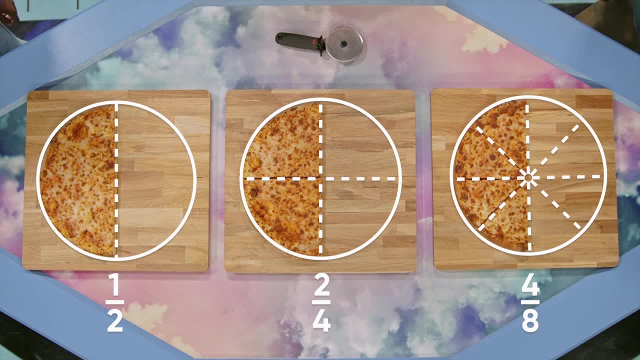 So who has more pizza left? We all have the same amount of pizza. Since yours was cut into two pieces, there's one left. Since this one was cut into four pieces, there are two left, And this one was cut into eight pieces, so there are four left. 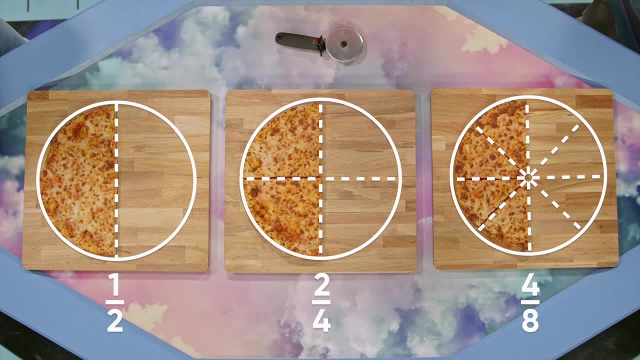 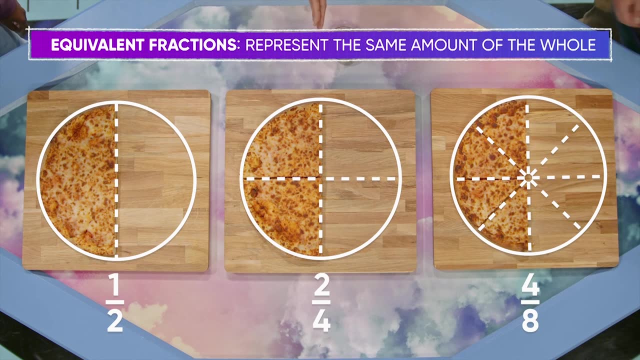 So, even though all these fractions have different numerators and denominators, they all represent the same amount of a whole pizza. Exactly, We call these equivalent fractions, which means they represent the same amount of the whole. The word equivalent means equal. So, since 1⁄2 equals 2⁴, which equals 4⁸, 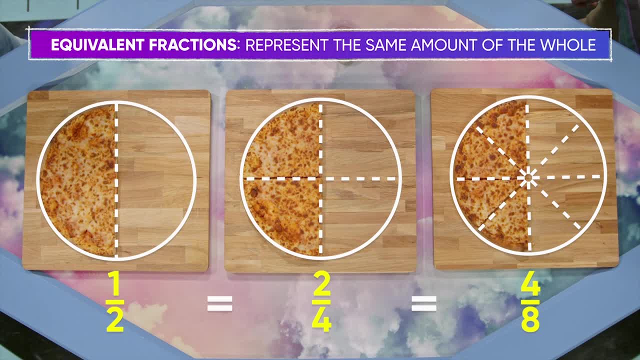 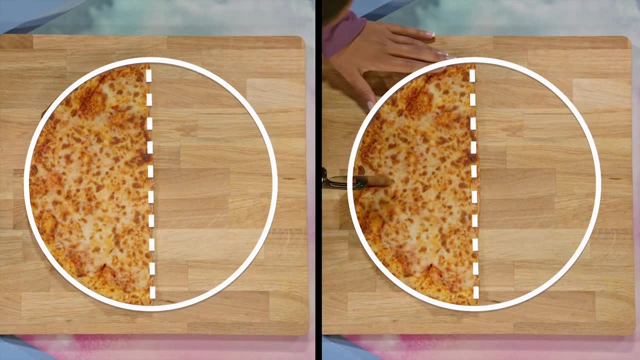 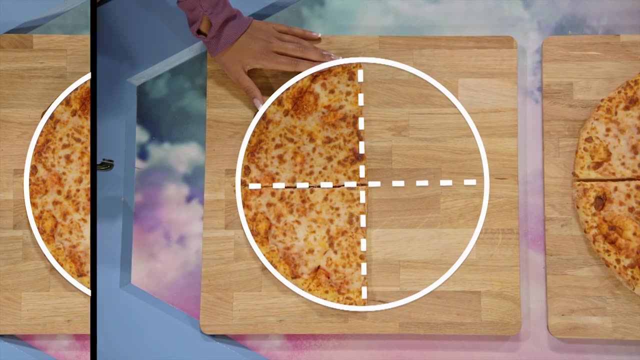 we can say they are all equivalent fractions. You're right. How could you prove that? by using this pizza cutter. If we double the number of slices in April's pizza, we can turn 1⁄2 into 2⁴. And if we double the number of slices again, 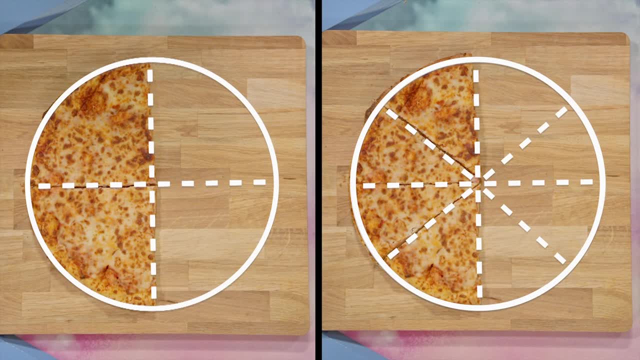 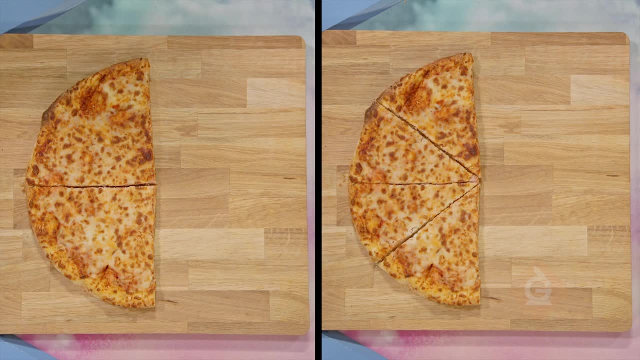 we can turn 2⁴ into 4⁸. That's right. When we cut them, we didn't change the amount of pizza we have left. We simply changed the number of slices that make up a whole. Hey, kids. 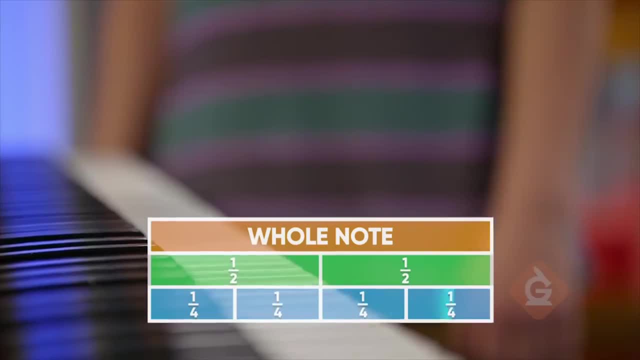 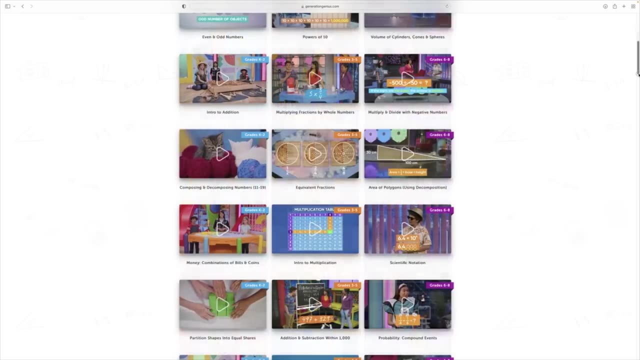 If you want to watch this whole episode and more, tell your teacher to sign up at GenerationGeniuscom. We cover all math topics, grades K through 8, and you get to watch it in class, but only if you tell your teacher. Captioned by Cotter Captioning Services.